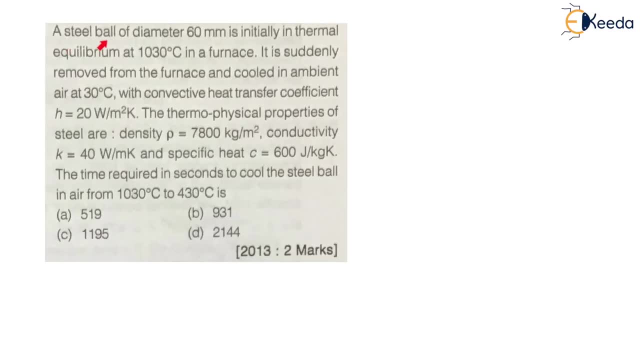 So let us understand the question. The question is a steel ball of diameter 60 mm. Now here they have mentioned it is a steel ball and ball is always spherical. So let us draw here. Let us say this is a steel ball. 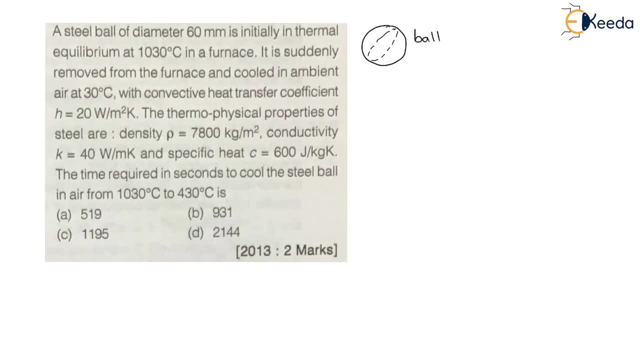 It is a sphere. Ball means always sphere having diameter 60 mm. Now, as diameter is given 60 mm, let us convert into meter. Therefore 60 into 10, to the power minus 3 meter. Then a steel ball of diameter 60 mm is initially in thermal equilibrium at 1030 degree Celsius in a furnace. 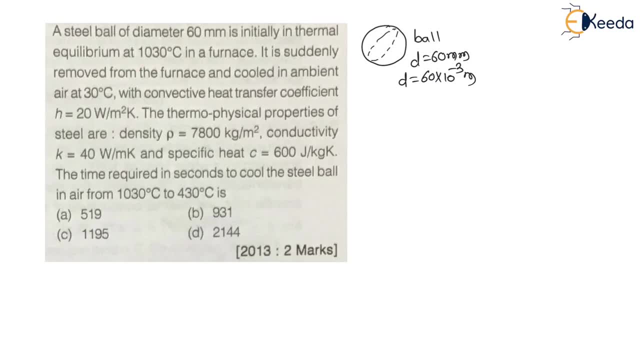 Means initial temperature of this steel ball is given. Therefore, this Ti initial temperature of steel ball is 1030 degree Celsius. Then it is suddenly removed from the furnace and cooled in an ambient air at 30 degree Celsius. Now this ball is taken into ambient air which is at temperature 30 degree Celsius. 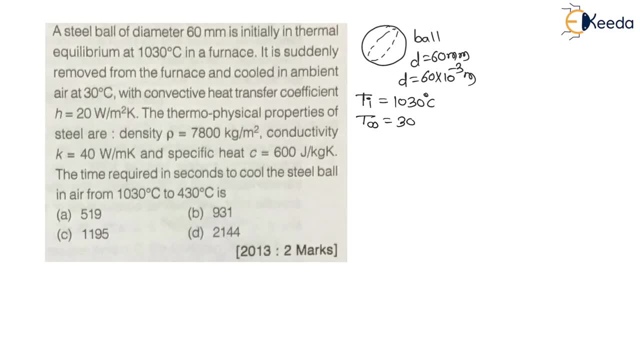 Means it is a surrounding fluid temperature, which is T infinity 30 degree Celsius. Then with convective heat transfer coefficient h, e. Now here convective heat transfer coefficient of air is given. h is equal to 20 Watt per meter square Kelvin. 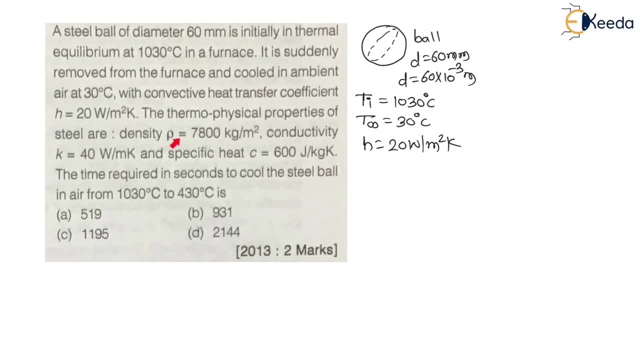 Then the thermophysical properties of steel are Now here. density of steel is given. Thermal conductivity, K, is given. Specific heat, C, is given. No need to write Here, written here. The time required in second to cool the steel ball in a year from 1030 degree Celsius to 430 degree Celsius is. 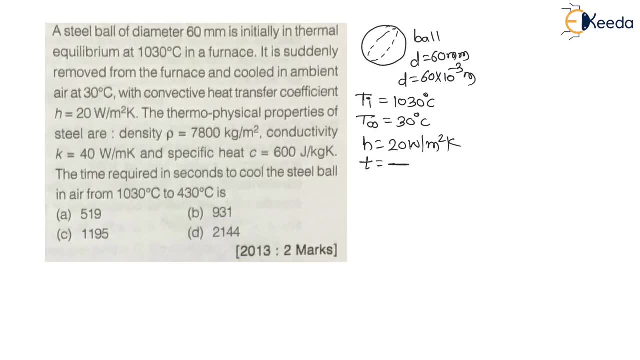 Now here: what is the time required to cool down? in second, They are asking in second, In second Right, To cool down this steel ball from 1030 degree Celsius to 430 degree Celsius. Therefore, the final temperature of steel ball is 430 degree Celsius. 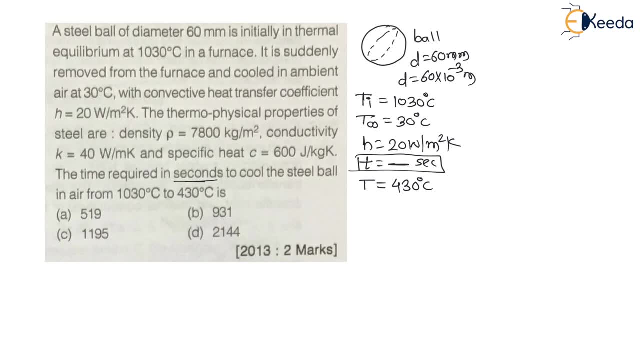 And to come from 1030 to 430,. what is the time required To solve this type of question? first of all, we have to find Biot number. The formula is nothing but H, L divided by K, Where L is characteristic dimension, which is volume divided by surface area of this sphere. 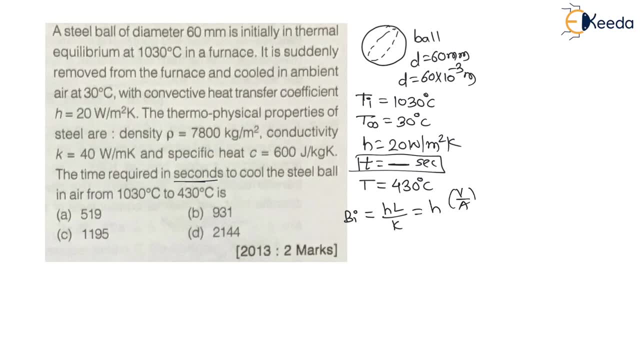 Therefore, I can write: is equal to H into volume divided by surface area of sphere divided by K. Therefore this Biot number becomes equal to H. Volume of sphere is 4 by 3 pi r cube divided by surface area is 4 pi r square divided by K. 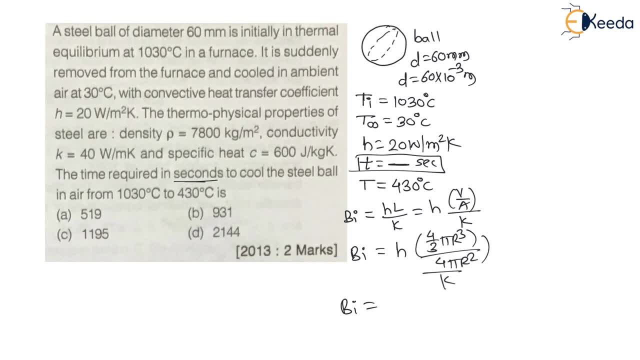 Right, So let us find this value. Therefore, my dear students, here we can say: the 4 pi r square will get cancelled And the resulting formula of Biot number will become: Biot number is equal to H r divided by 3 K. 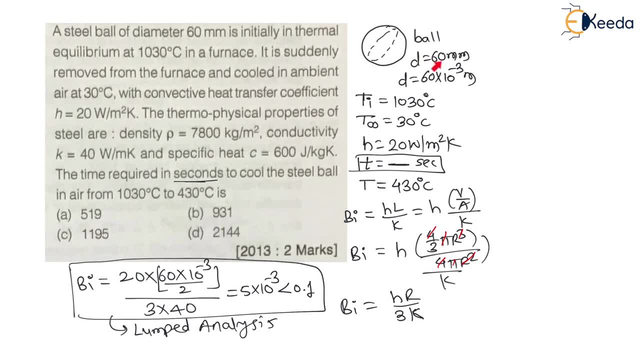 Here. if I put the values, H is nothing but 20.. r is diameter divided by 2.. Therefore, 60 into 10 to the power minus 3 divided by 2.. Now, 3 into K is 40.. 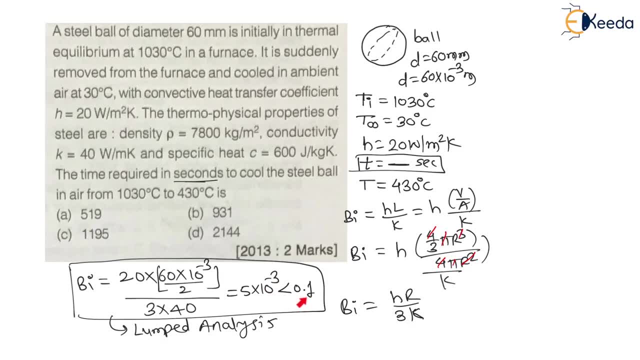 Then I will get Biot number is 5 into 10 to the power minus 3, which is less than 0.1.. As this is less than 0.1. Therefore, lump analysis is valid. That is T minus T, infinity. 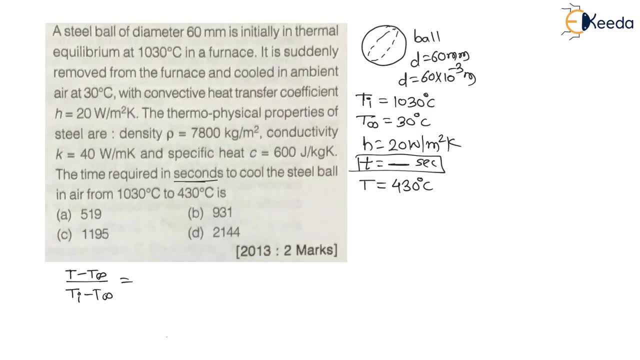 They have a T i minus T, infinity is equal to e, to the power minus H, a. They have a rho v c p into time T, Right? This formula is now useful to solve this question. Now, my dear students, where capital T is the temperature after time T, 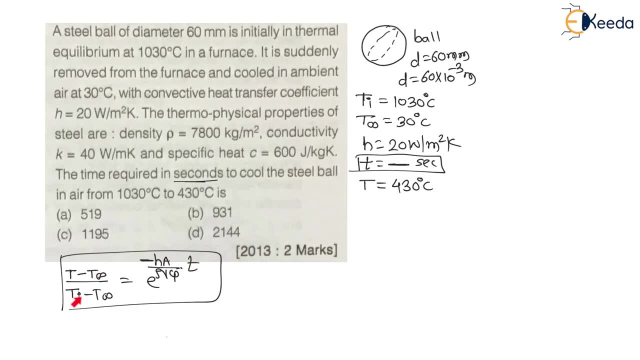 T infinity is surrounding fluid temperature. T i is initial temperature of the steel ball. H is convective transfer coefficient. A is the surface area of this steel ball which is in contact with the air. Rho is the density of steel ball. V is the volume of this steel ball. 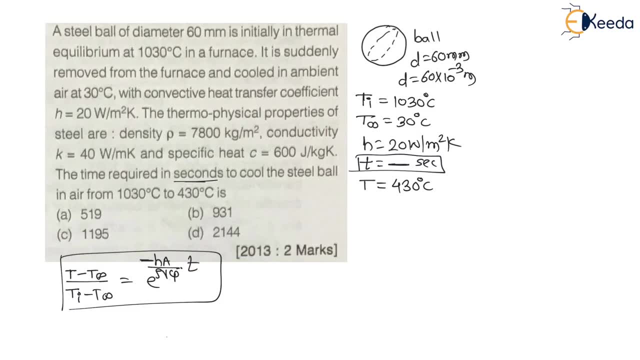 Cp is specific heat And T is the time, Right Now, my dear students, as it is spherical object. Therefore, what is area by volume ratio of sphere? Area divided by volume ratio? Now, for this sphere, the surface area is 4 pi R square. 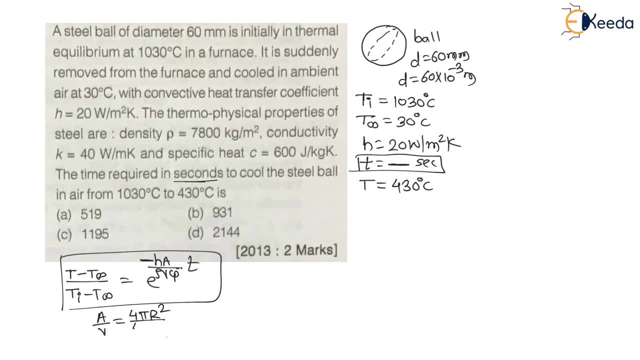 It is 4 pi R square. Volume is 4 by 3 pi R cube, Right. So here this 4, 4 will get cancelled. Pi pi will get cancelled. R square- R square will get cancelled. It will become 3 by R. 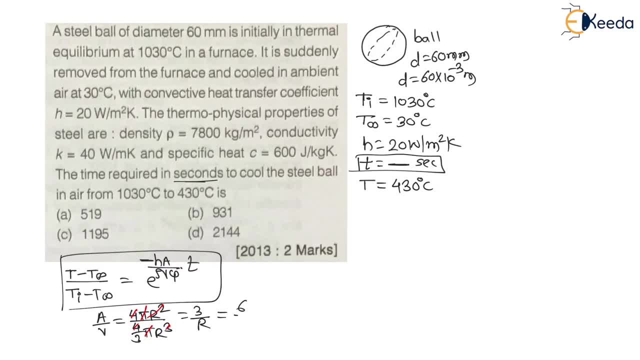 It will become 3 by R. Therefore, again can I write 6 by D, Right? Therefore, this area divided by volume, Area divided by volume, we can replace with 6 divided by D. So we will replace with 6 divided by D. 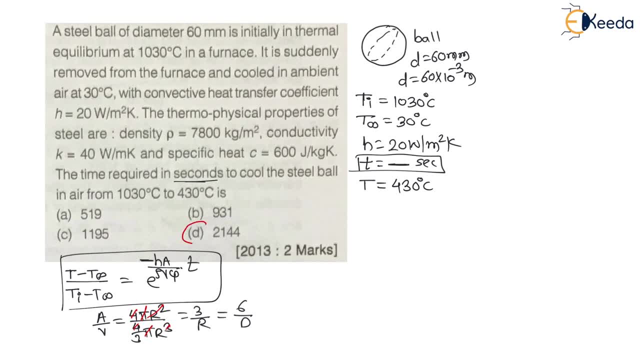 Right Now, here, I will tell you answer. The answer is option D, because I am going to erase this question. That's why I am telling you answer. Option D will be the correct choice, So let us erase this question, Right. 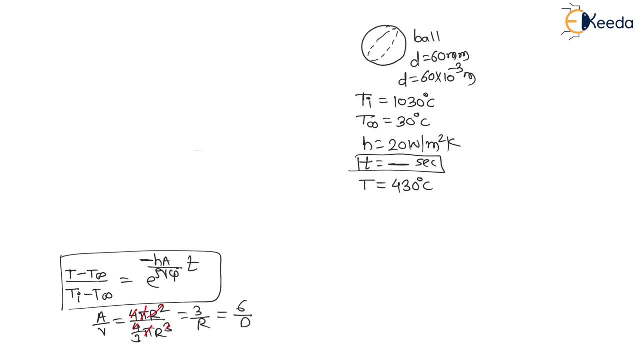 Now, let us solve this. Now, my dear students Here, if I replace A by V, by 6, by D, then the formula becomes T minus T infinity divided by TI minus T infinity is equal to E to the power, minus EH, minus EHT, divided by rho CP into. 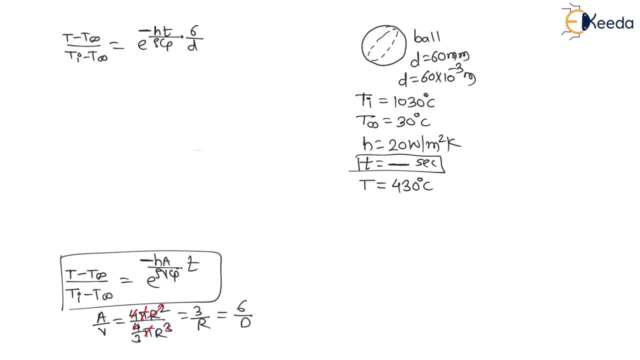 6 divided by diameter, D Right, Because area divided by volume becomes 6 divided by D. So let us put the values here. only Time is unknown. If I put the values, T is nothing but 430.. T infinity is 30 divided by TI is 1030. minus T infinity is 30 is equal to E to the power. 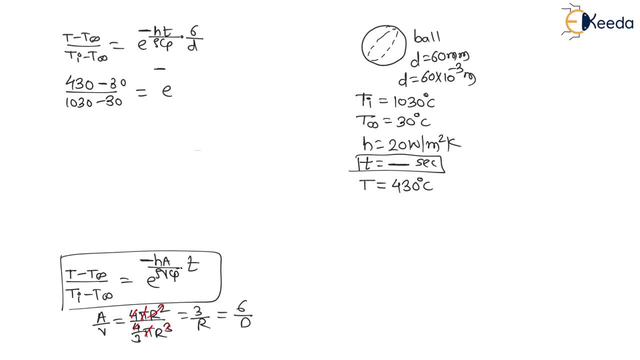 minus EH is nothing but convective transfer coefficient. Now this EH value is given 20.. Right, Let us remember It is written in the question. Then time we have to calculate into 6. divided by Now, density was given. 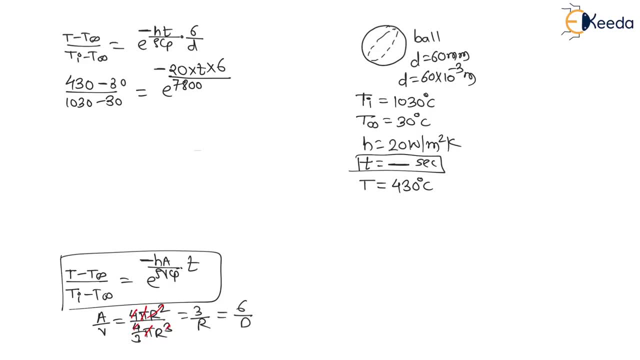 Density is 7800.. You have question In question. it is written: Density is 7800.. Right Into CP, Now specific it, That is, C is given 600.. You can check question. Into diameter: Diameter is given 60 into 10 to the power minus P. 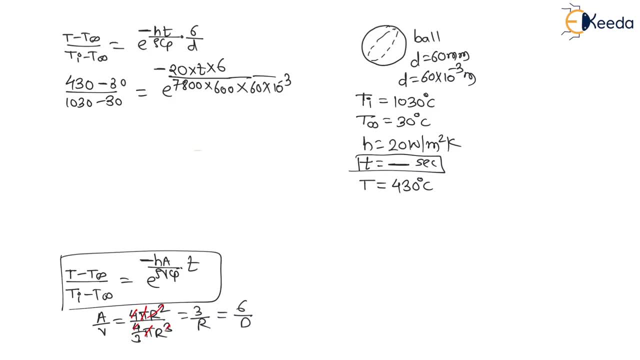 Right Now, my dear students, The equation will become again: This will be 400 divided by 1000.. This is equal to E to the power minus 4.27 P. 5 into 10 to the power minus 4 P. 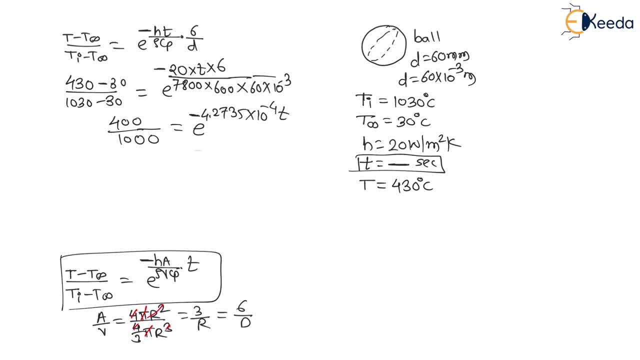 Now if I consider LN function on both side, That is, log to the base E, Then this exponential function will go. Therefore I can say LN of this will become: 4 divided by 10 is equal to minus 4.27. P 5 into 10 to the power, minus 4 into T.